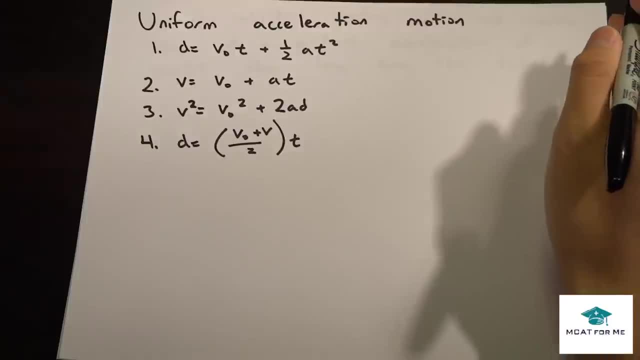 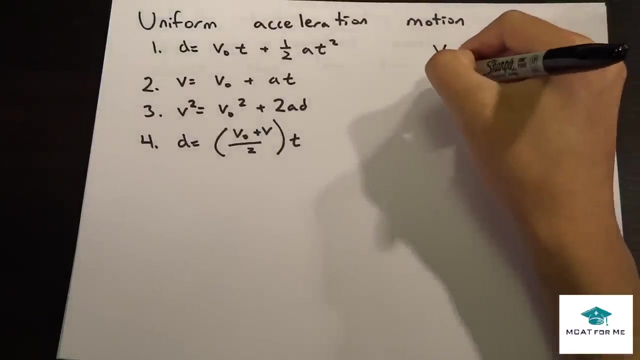 So, for example, this one: what isn't given? Well, we know that the final velocity v final is not given, Okay, and so that's important to know, because it's important to know which was not given. So we know which equation we use, because they will only give us a certain amount of information, And whichever one they don't give us, we know that that's the equation that we're going to be using. In this one we aren't given d, in this one we aren't given t, And in this one we aren't given a. So it has all the. 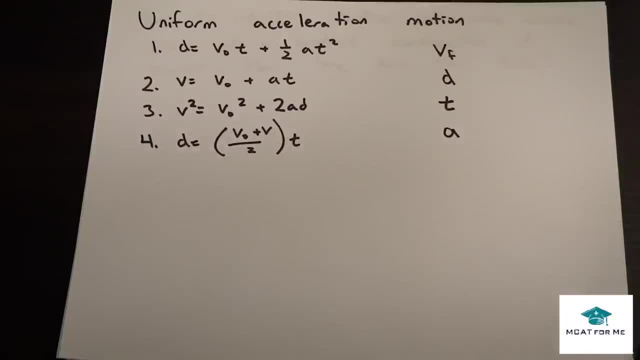 four of our variables covered. so, for example, if they give us everything except the time, we know that, we use equation three. they give us everything except acceleration, we use equation four. so these equations will be very, very useful for us, and so we'll just start off with an example. so an individual 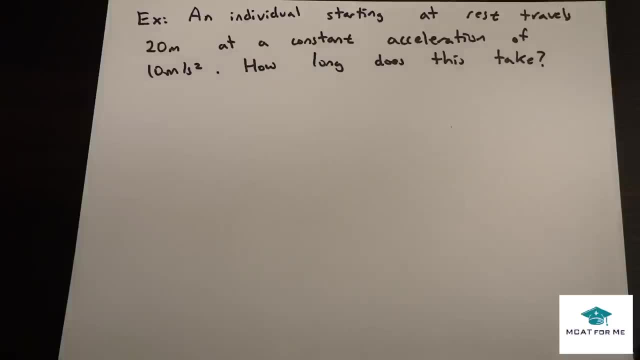 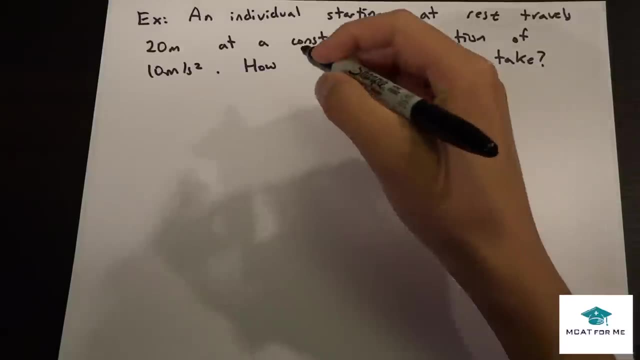 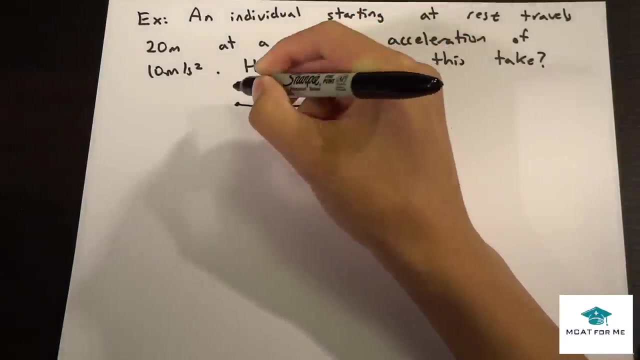 starting at rest, travels 20 meters at a constant acceleration of 10 meters per second. squared, how long does this take? so the first thing we want to do for these types of questions: we could draw a picture. it's not gonna help us too much, but so he starts from rest. so he starts with a V naught at rest and he goes for a. 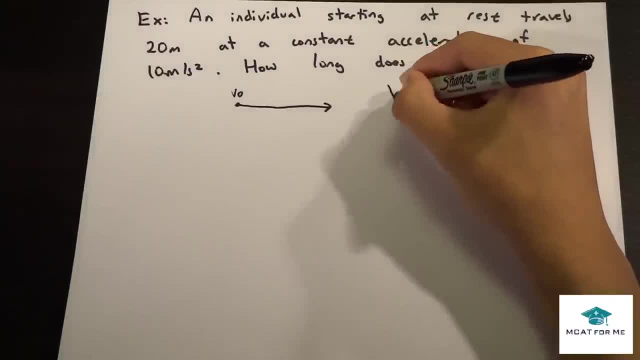 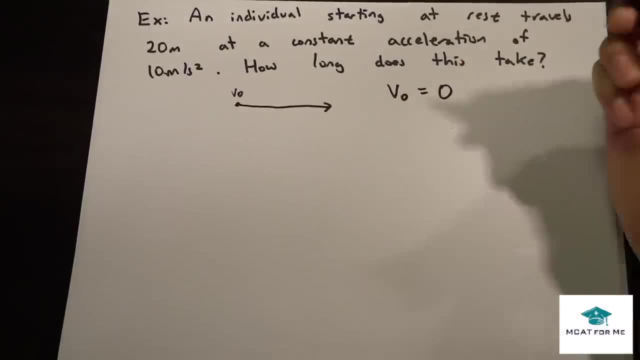 certain distance, how long does it take? so that's not really important to us. what we need to know are the variables involved. so V naught is what? zero right, because he starts from rest, he travels 20 meters. so that's: D equals 20 at a. 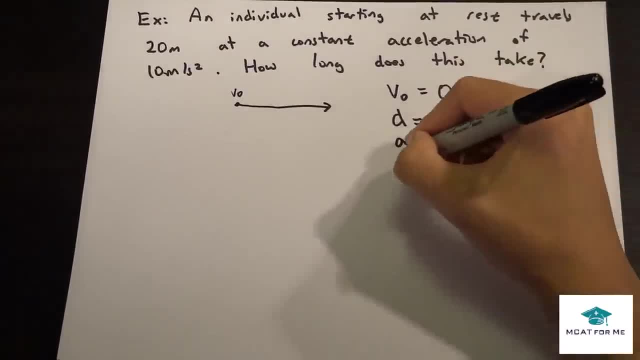 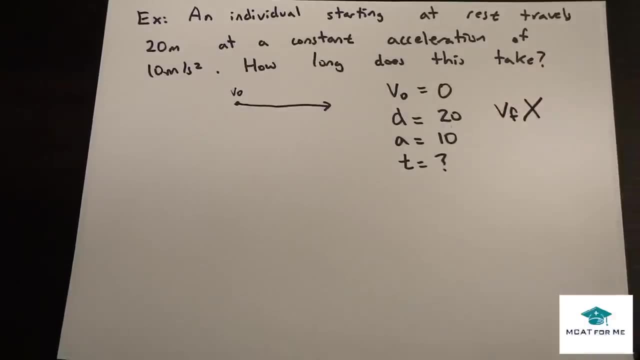 constant acceleration of 10. okay, so in this example, we guys want to write t, we want to write to stay at zero, right, we want to find T. but what didn't they give us? well, it didn't give us V final, so we were never given V final. so if we look back at our equation, 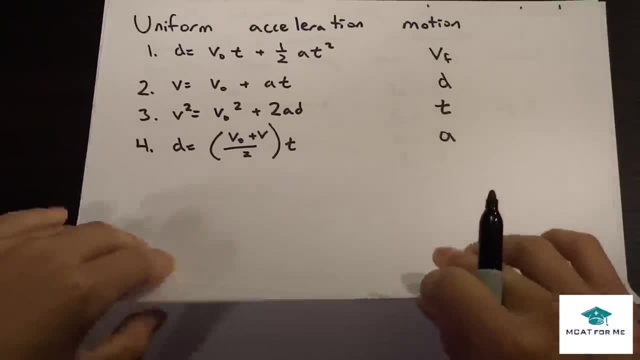 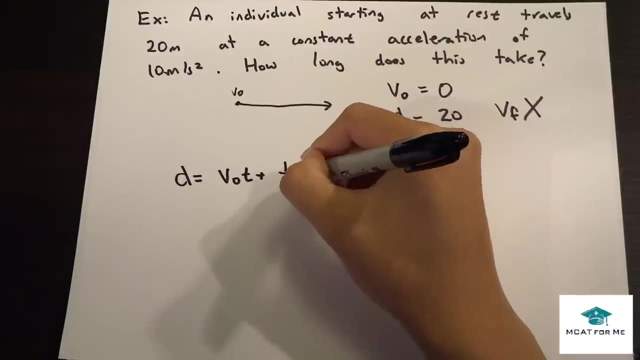 if we're not given V finals of, we use the first equation right there. all right, so the equation that we use is D equals V, not T plus one half at squared. all right, then we just plug stuff in. okay, so z is one half a trigonometric eight. what we can do is: all right, then we just plug stuff in: z equal and z Worcester speed. all right, so Z is one half a T squared. all right, they would just thoughts o.